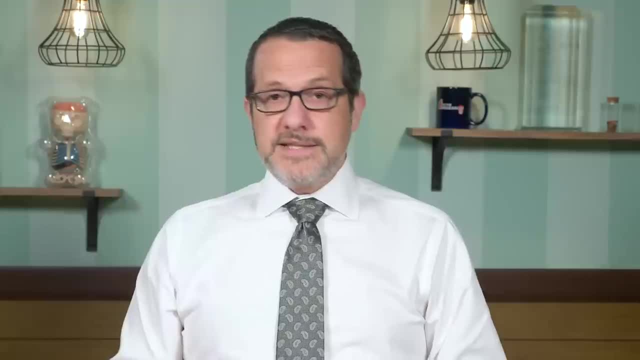 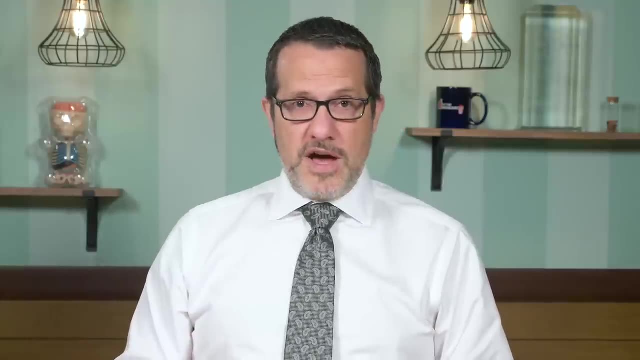 and are promoted by some health officials as well as some countries. Research, however, suggests that warnings about sitting at work are overblown and that standing desks are overrated as a way to improve health. That's the topic of this week's Healthcare Triage. 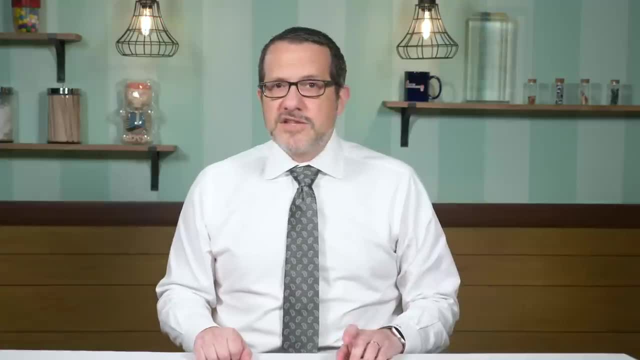 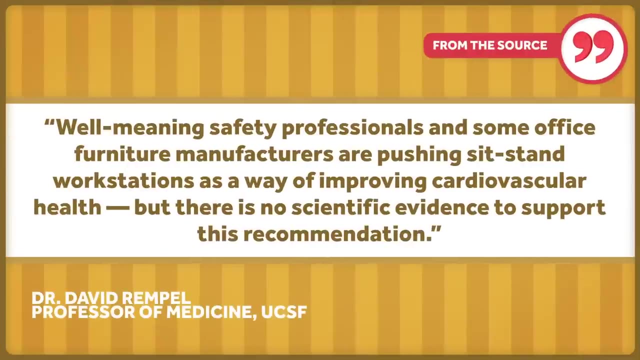 Dr David Rempel, a professor of medicine at the University of California, San Francisco, who's written on this issue, said to me in an email, and I'm quoting: Well-meaning safety professionals and some office furniture manufacturers are pushing. 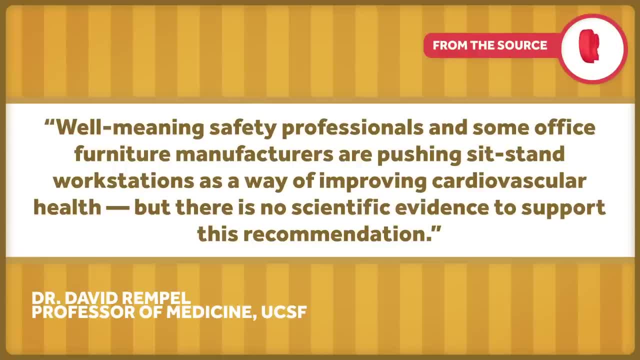 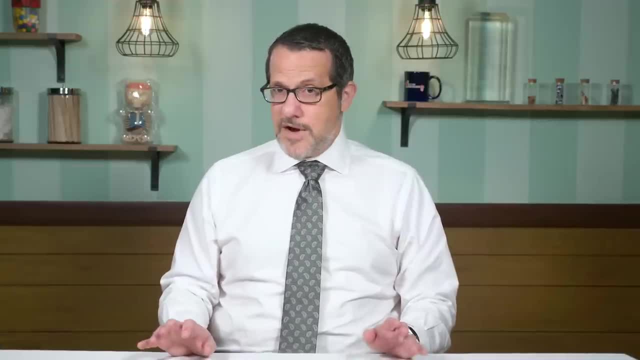 sit-stand workstations as a way of improving cardiovascular health, but there's no scientific evidence to support this recommendation For convenience and comfort. it's nice to have options if you have various aches and pains. Alternating standing and sitting while using a computer may be useful. 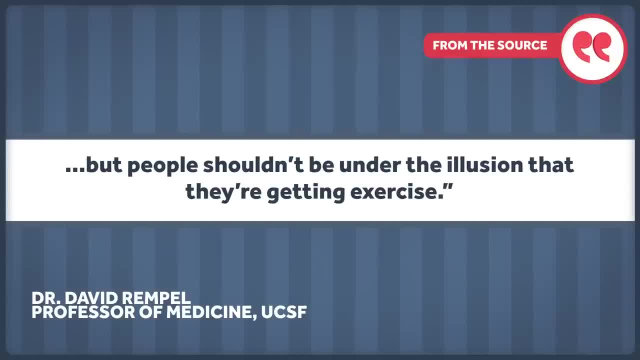 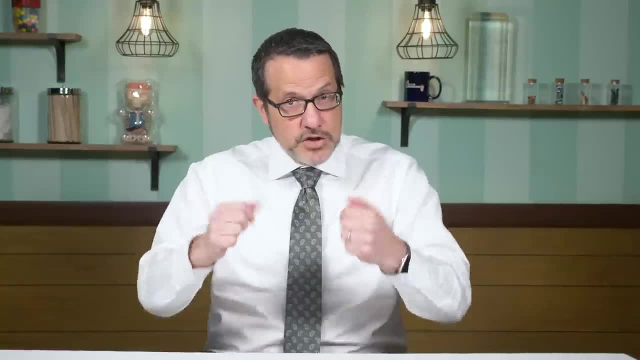 for some people with low back or neck pain, but people shouldn't be under the illusion that they're getting exercise. Let's start with what we know about research on sitting, then explain why it could be misleading as it relates to work. A number of studies have found a significant association between prolonged sitting time. 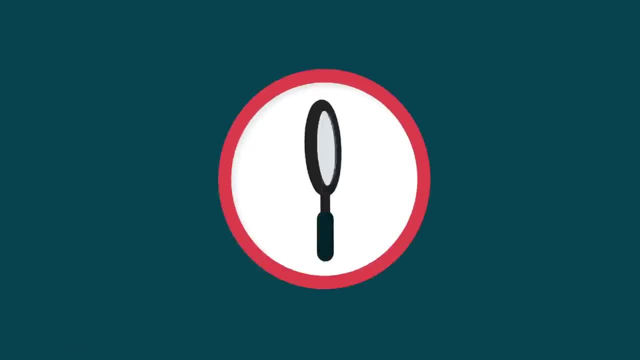 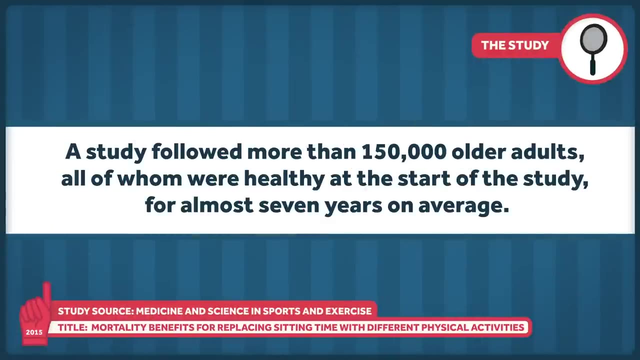 over a 24-hour period and increased risk for cardiovascular disease. A 2015 study, for instance, followed more than 150,000 older adults, all of whom were healthy at the start of the study, for almost seven years on average. Researchers believe that sitting at work is a way to improve cardiovascular health. 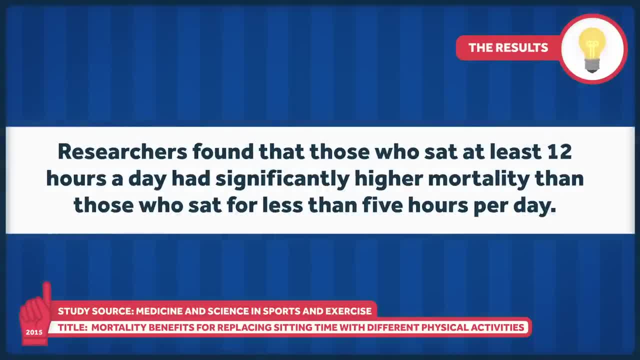 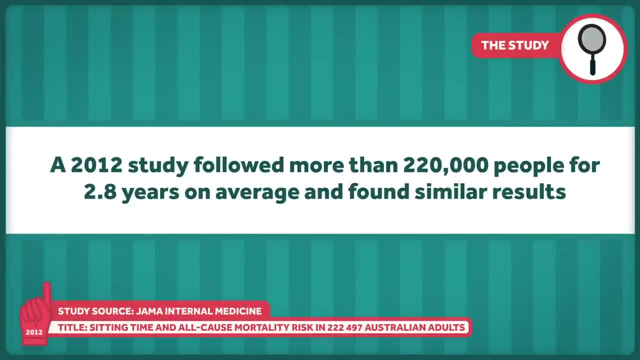 and they found that those who sat at least 12 hours a day had significantly higher mortality than those who sat for less than five hours per day. A 2012 study in JAMA Internal Medicine followed more than 220,000 people for 2.8 years on average. 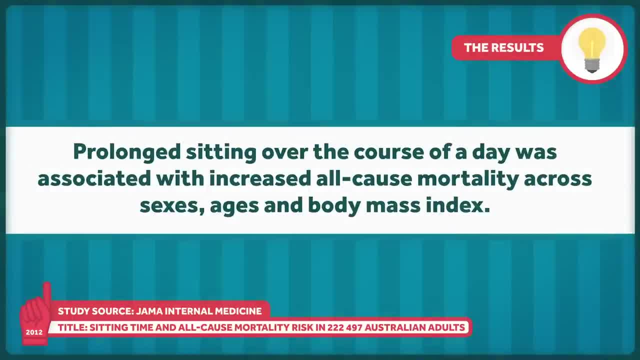 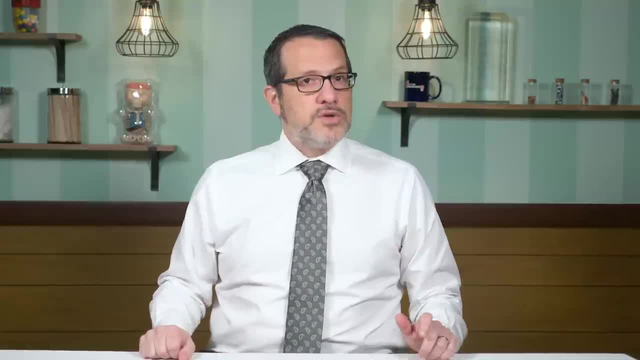 and found similar results. Prolonged sitting over the course of a day was associated with increased all-cause mortality across sexes, ages and body mass indexes. So did a smaller but longer study published in 2015 in the Journal of Physical 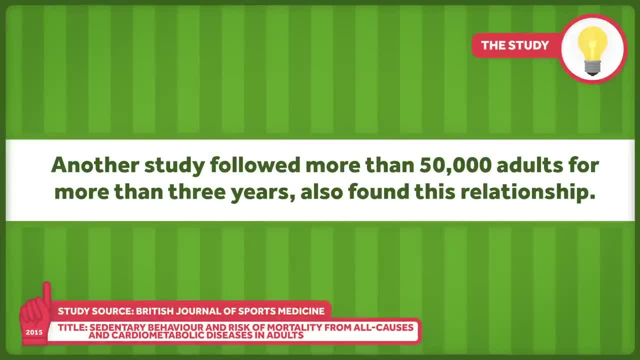 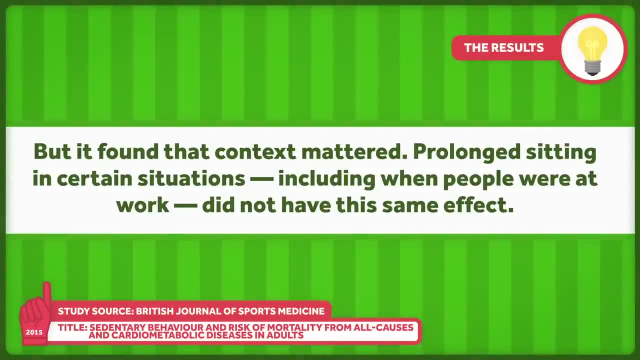 Activity and Health. Another study from 2015,, which followed more than 50,000 adults for more than three years, also found this relationship, But it found that context mattered. Prolonged sitting in certain situations, including when people were at work. 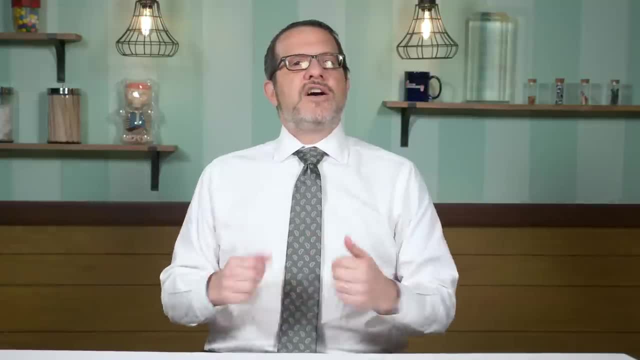 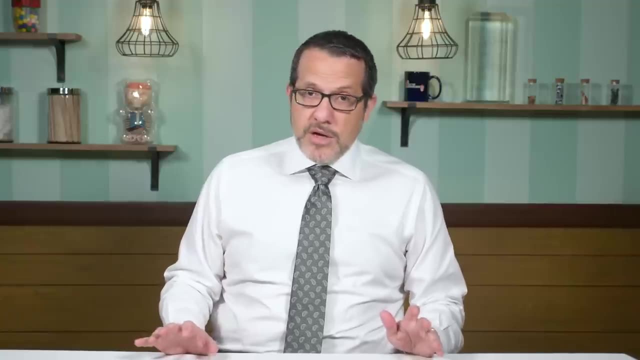 didn't have the same effect. Why might that be? Sitting itself may not be the problem. It may be a marker for other risk factors that would be associated with higher mortality. Unemployed or poorer people, who would also be more likely to have higher mortality, may be more. 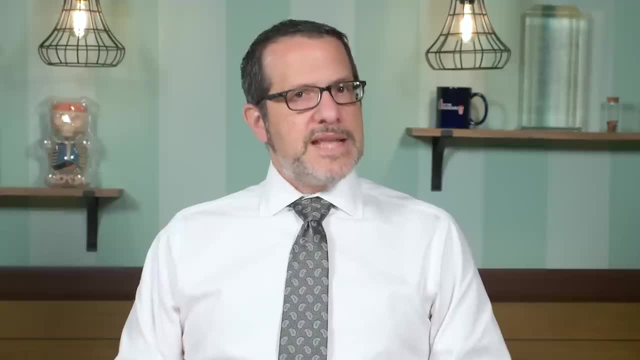 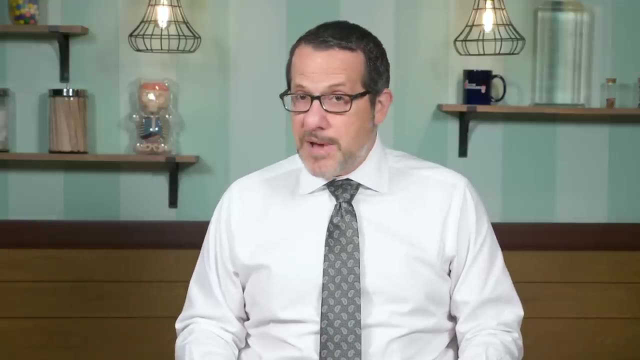 likely to spend large amounts of time sitting at home. For some, sedentary time is a marker, not the cause, of bad outcomes. Studies looking specifically at work don't find a causal pattern. One 2015 paper focused on workers aged 50 to 74 in Japan for more than 10 years on average. 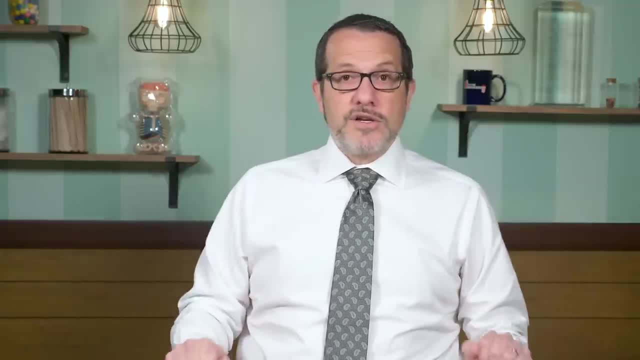 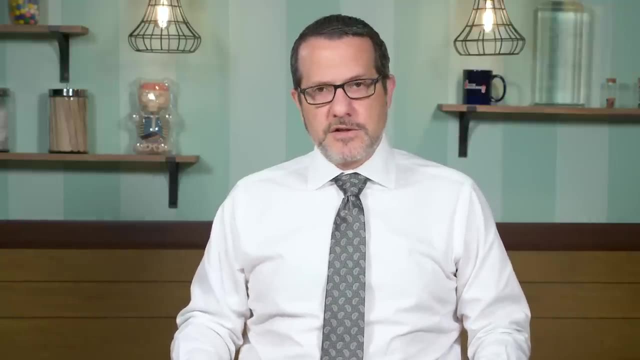 per participant. It found that among salaried workers, professionals and those in home businesses, there was no association between sitting at work and cardiovascular risk. A 2016 study found that the average age of people sitting at home was about 50 to 74.. 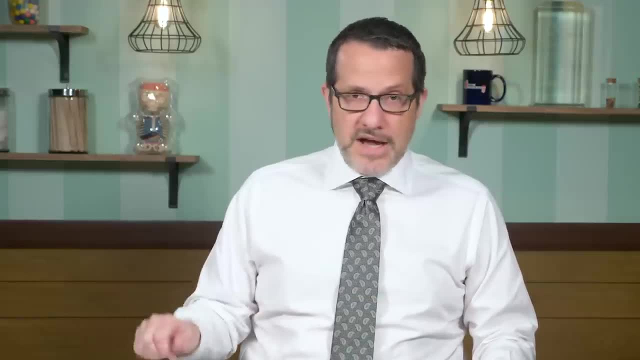 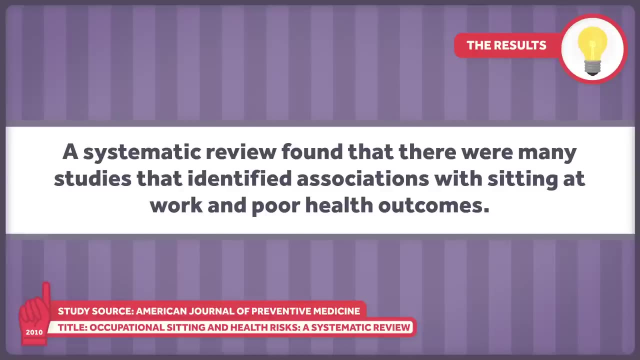 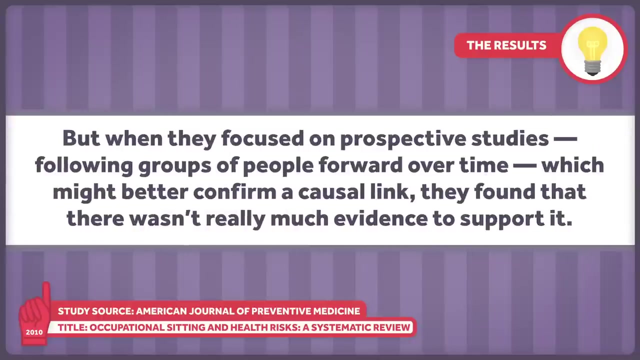 A 2016 study examining Danish workers also failed to find a link. A systematic review published in the American Journal of Preventive Medicine found that there were many studies that identified associations with sitting at work and poor health outcomes, But when they focused on prospective studies following groups of people forward over time. 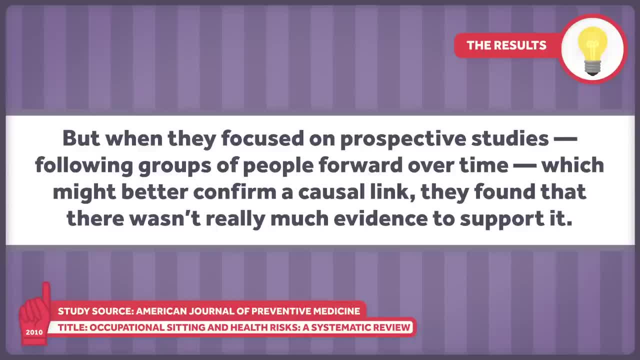 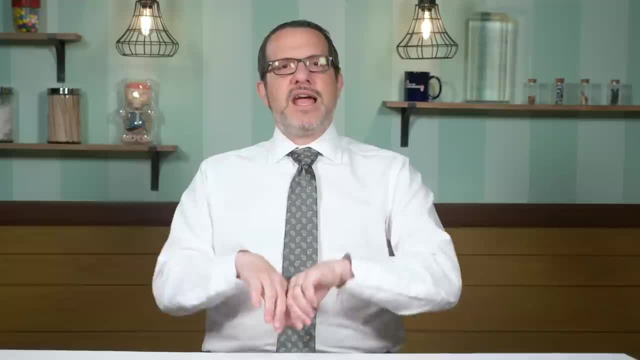 which might better confirm a causal link. they found that there wasn't really much evidence to support it. Moreover, these studies tend to focus only on the positive effects of standing at work and the negative effects of sitting. A full accounting would also examine the opposite. 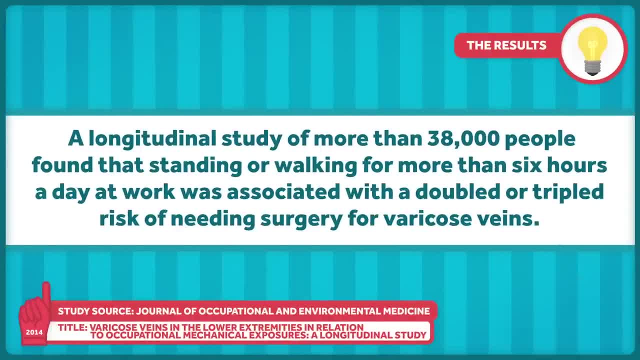 A longitudinal study of more than 38,000 people published in the journal Occupational and Environmental Medicine found that standing or walking for more than six hours a day at work was associated with a doubled or tripled risk of needing surgery for varicose veins. 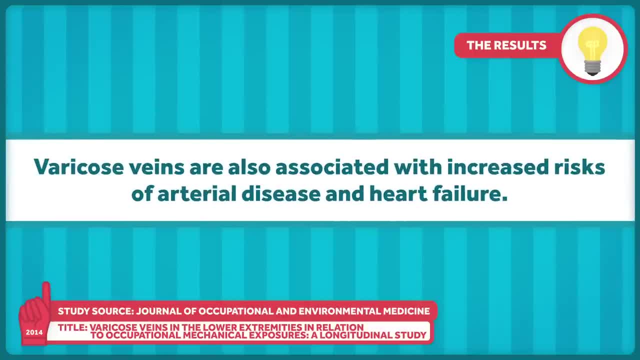 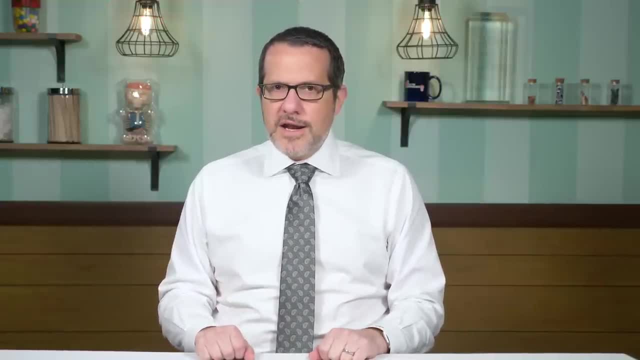 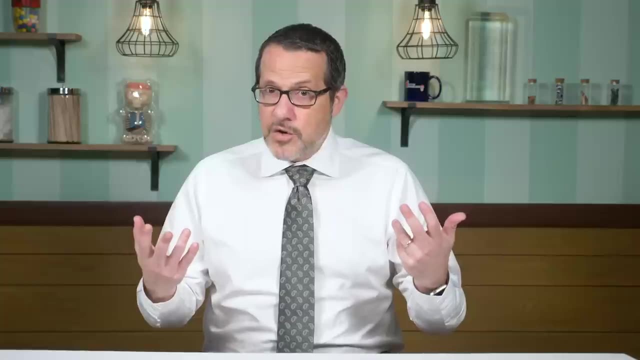 Varicose veins are also associated with increased risks of arterial disease and heart failure. It's possible, though, that standing at work, as with sitting too much at home, could be a marker for other unhealthy demographic factors or health risks. There is a difference between those who must stand or walk for most of the workday and those 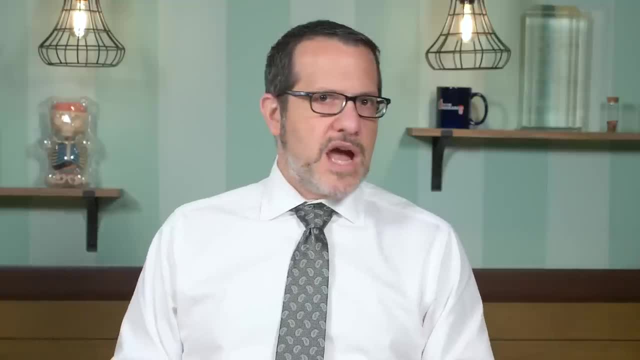 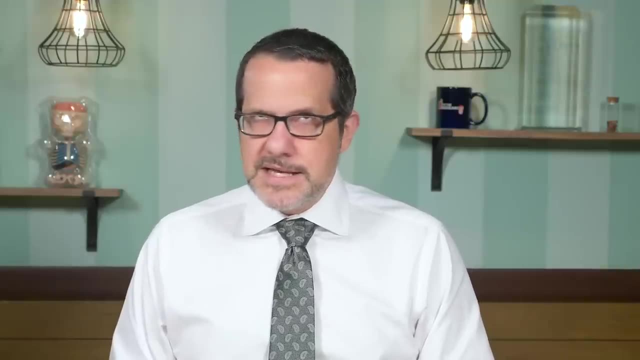 who can sit at any time, But particularly for those who don't have the option to lower their desk. there is at least some evidence in that study and in others that standing for much of a workday is not helpful. A number of countries have called for more standing and less sitting at work.